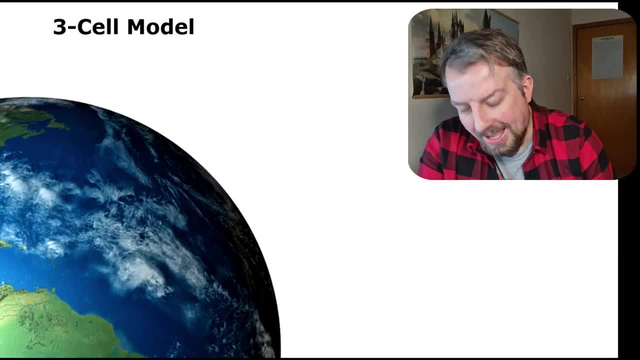 is redistributed. We have our sun away over here somewhere again- not small, just very far away- and the light comes down and hits the equator. So what we're going to do first of all today is we're going to pop our equator in, just so we know roughly where we're looking. 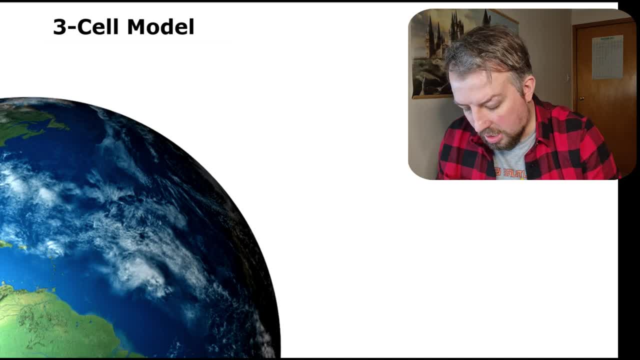 and we're going to look at the temperature. So we're going to look at the temperature and we're going to pop our equator in and then it gives us a working point. So we've got an equator there. Probably what else we want to add into our diagram around is just our atmosphere to give us. 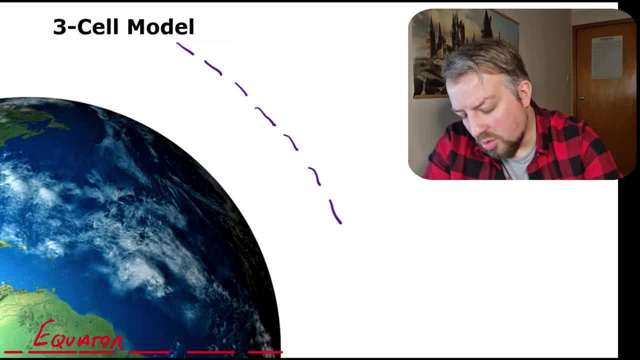 some context about where this is, and I'm not saying a whole atmosphere. this is really just going to be the troposphere, which is where most of our weather patterns happen. So at the equator, we've said before, we have a surplus of energy, an excess of energy, that is. 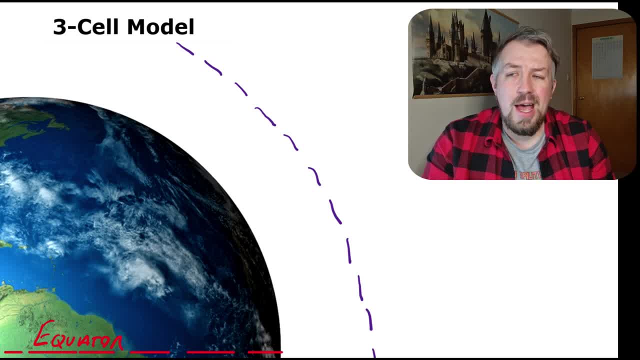 making the air warmer, making the water and the land warmer, and what happens when that occurs is that air starts to rise. So at the equator we have rising air, and this is known as low pressure. So this is a low pressure zone, where air is starting to rise, but when it reaches the ceiling of this, 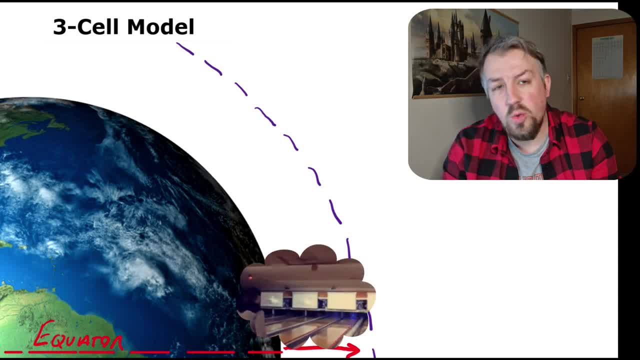 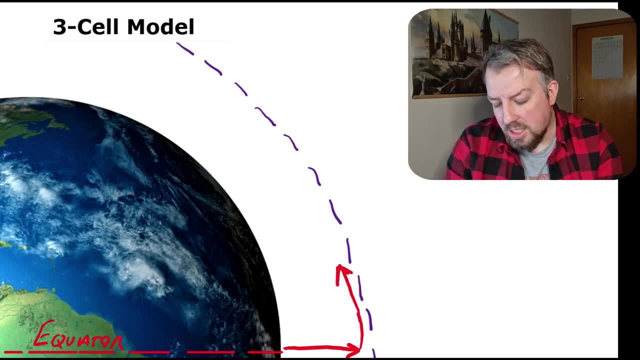 troposphere. what happens then is that the air starts to rise. and the air starts to rise and the temperature rises, and the air starts to drop down and the temperature rises, and then it actually doesn't go any higher. so it's pushed out to the side and it's pushed away north, and once it gets, far enough north. it actually then starts to cool and as it cools it begins to sink back down and again can't sink any lower than the planet. so it's actually then forced back south, where it slowly warms up again and joins in to the warm area, which then moves it back north. 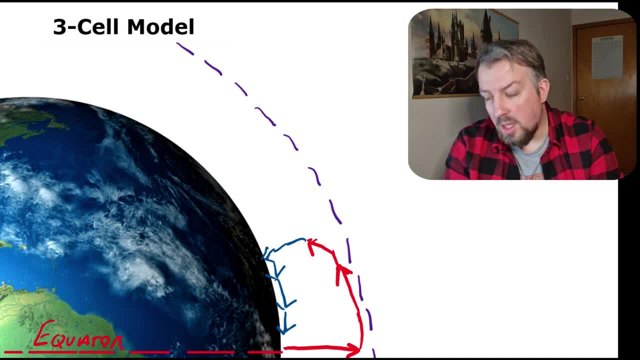 so this is going to be number one. this has then created an air cell where we'll get this low pressure that comes up, moves north and then sinks and returns to the equator, creating what's called the Hadley cell. and now this is driven by the temperature, by this excess of heat equator. 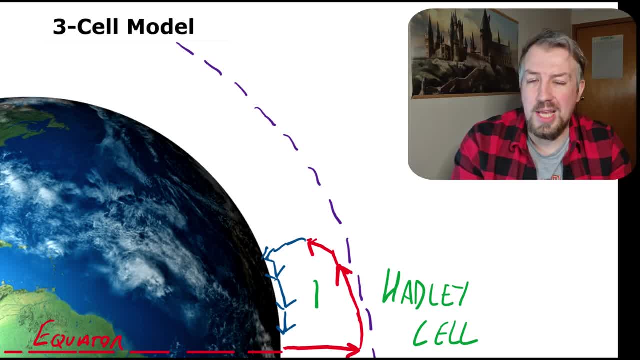 that creates air pushing up and then moves north. the opposite occurs at the poles. because the poles are colder, they make the air sink and they make it drop down. so if we take our air at the poles and push it straight down, this is called high pressure. if you think about it, the air is heavy. 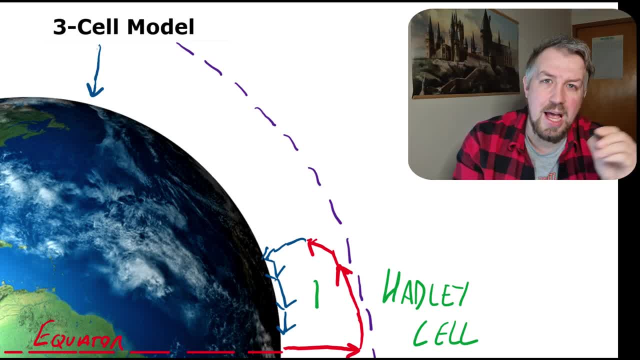 it's getting, it's sinking and as that eight, that heavy high, is going downwards. now it's a complete opposite to our Hadley cell, where the main driver in our Hadley cell is the fact that the air is being warmed at the equator. this time the air has been cooled at the poles and sinking it down. but 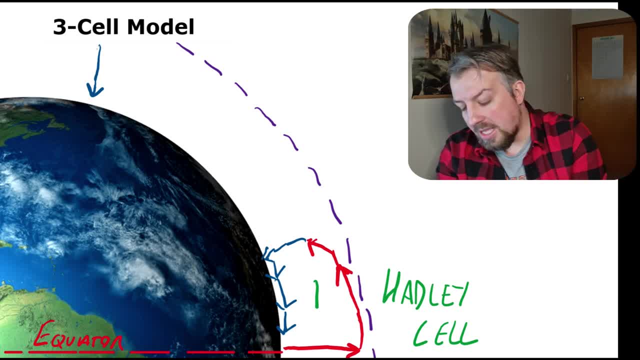 again. it can only sink so far as the surface of the earth. then it is deflected south. it would actually happen this side as well, where it's deflected so here. but we're looking primarily at just the one section, the cross sections now. so it's then deflected south until 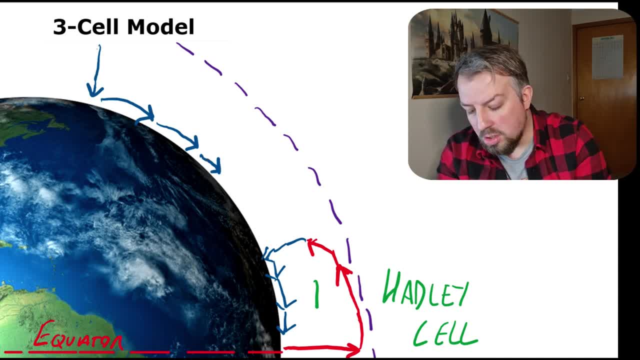 the same thing occurs: that it gets warmer. now it's round, happens around about 60 degrees north, and it gets warm enough that it then rises back into the air atmosphere and is then deflected north again, where it cools and sinks back to the earth. now this is our second cell. 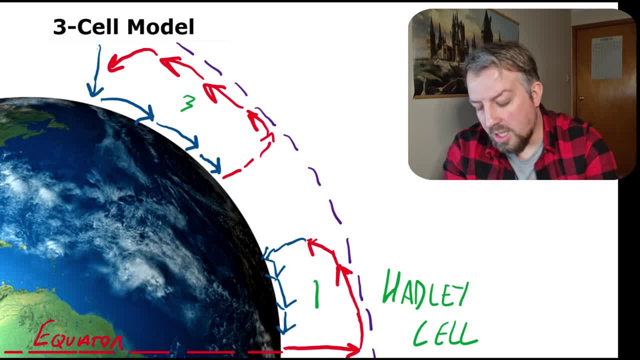 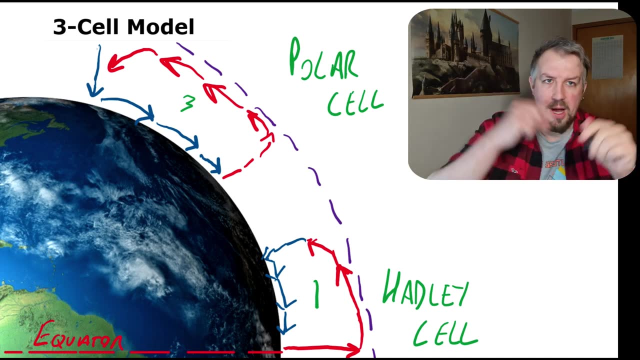 but because we've got one to go in the middle, actually can all this number three, and this is the polar cell named after the fact it's at the poles found in both north and south poles. it used to be that we only actually ever thought that these, these two and these were going back. 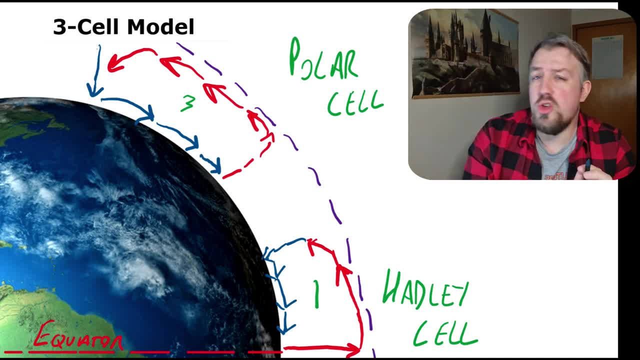 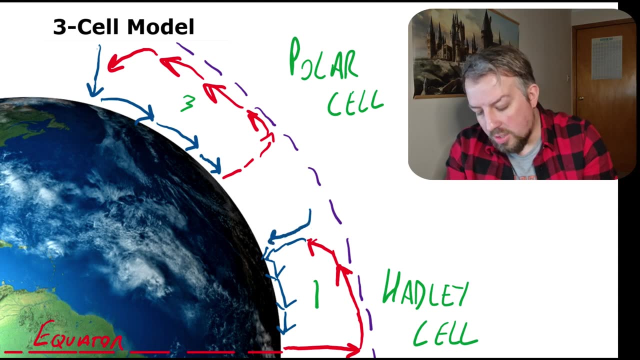 and forwards, um, but we actually have a third one. the third one is not driven by the temperature, it's actually driven by friction. as the Hadley cell is dropping down, it also pulls other air from it down with it as well and forces that away north and as the polar cell. 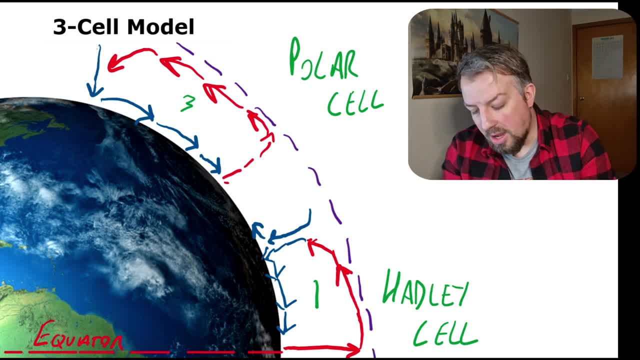 is rising north. it is actually pulling in air and forcing it upwards as well and it diverges and converges at these two other cells. so the Hadley cell goes. Hadley cell goes to about 30 degrees north and the polar cell drops down to about 60 degrees north. 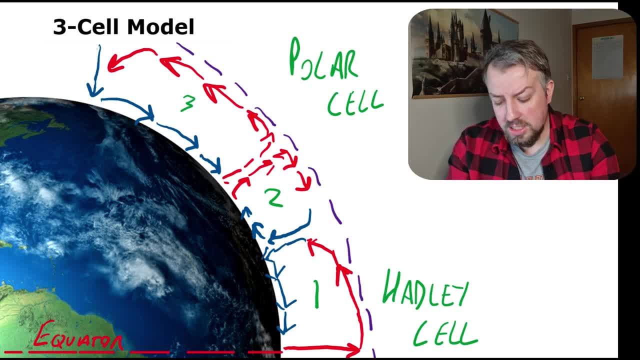 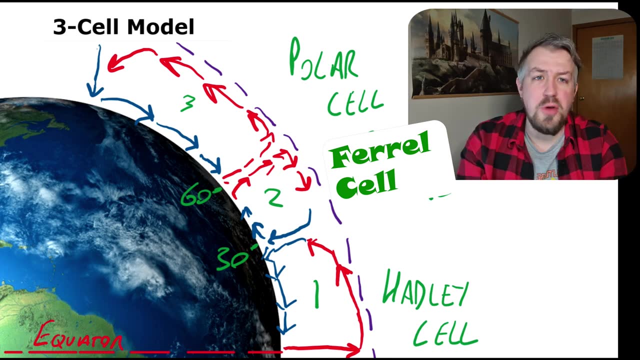 so between that 30 and 60 degrees, we actually have this third cell known as the ferro cell, and this is our three cell model. so we now have the Hadley cell, the ferro cell and the polar cell that all work together to actually distribute air. how does this actually even out our surplus? 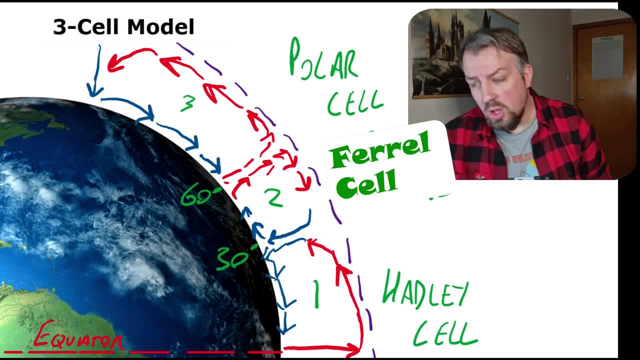 and our deficit that we see in our solar insulation. well, this air that's moving across the ground is not actually like imaginary, it's actually there. that is what wind is, and these are our surface winds, and our surface winds are actually moving air from one area to the 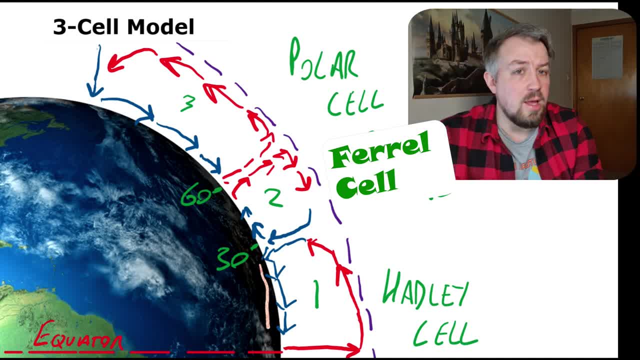 next. so if we bring in a little help, we might ask like princess poppy from trolls: so if she starts at the equator down here she could be like an air molecule that is carried up into the air and then transfers along and then sinks back down 30 degrees north. 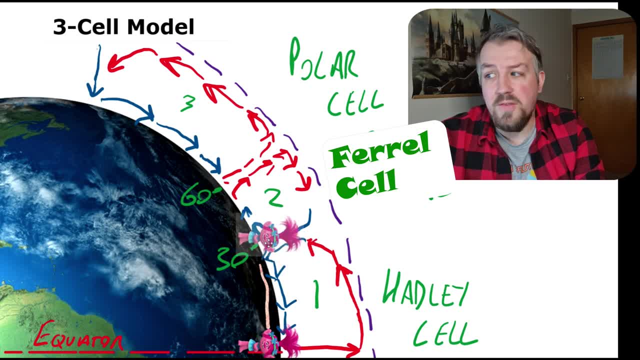 but instead of returning to the equator, she is then carried by the federal cell further north and then, 60 degrees north, she gets carried up into it again and then travels north to the poles, where we've got this warm energy from the equator. that's now. 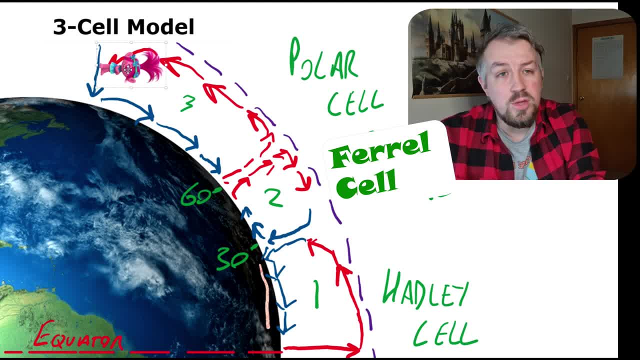 made all the way to the poles, and this is where we also then see the reverse, that if poppy is in at the poles, she's cooled down, she's really cold, and then travels south, is picked up by the fellow cell again, travels south, cools down, but this time travels back to the equator and 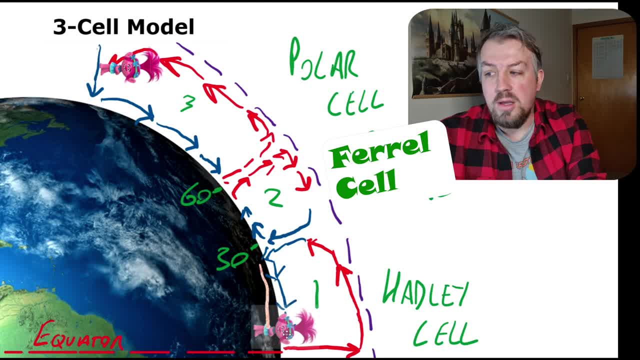 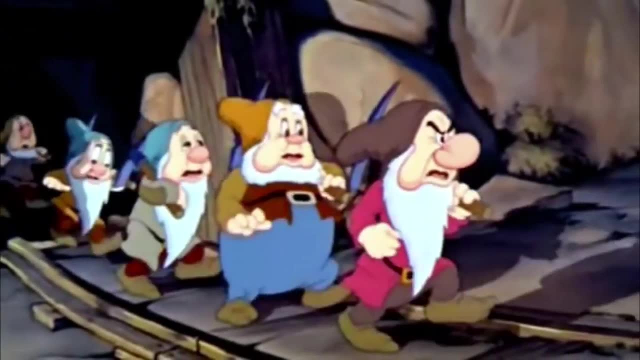 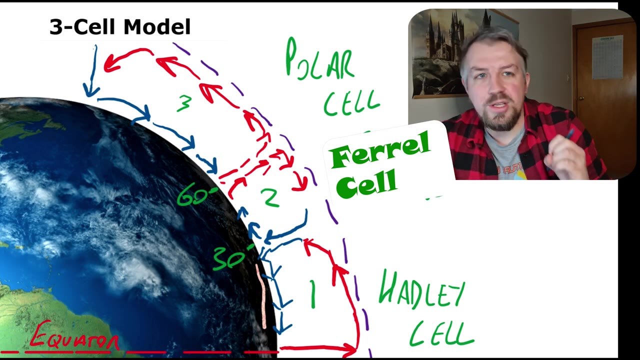 now we can see how cold air from the poles is traveled, is transferred back down to the equator. so easy way to remember this is: it goes high, low, high, low. it's off to the poles we go. and the one last thing to add into this is this is not just happening in a single cross section. 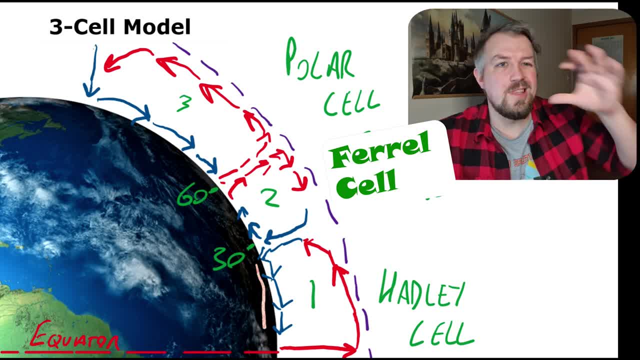 this is happening across the whole of our planet. this is a fully 3d object that is happening everywhere and it doesn't just happen in the whole of our planet, but it's happening in different places, linear way. these air, these surface areas are not just going up and down there, because our earth 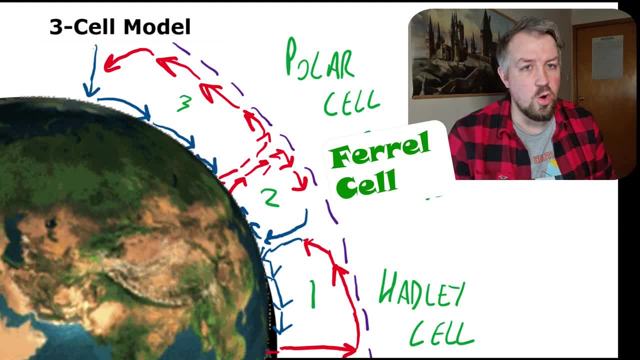 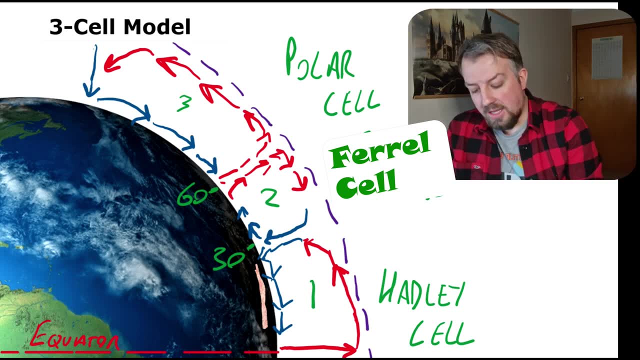 spins and it moves around. it actually deflects our winds around. so between this 30 degrees north and the equator our winds are actually deflected that way. so the winds in the northern hemisphere deflected to the right. between the north, the 30 and 60, the winds are deflected. that